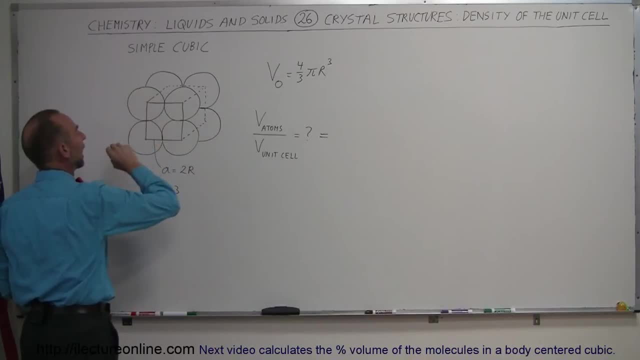 that would be four unit cells all containing a portion of that atom. and then you have another set of four unit cells right above it that would also contain a portion of that particular atom, in such a way that only one eighth of each of these atoms is contained within the unit cell. Notice, just this. 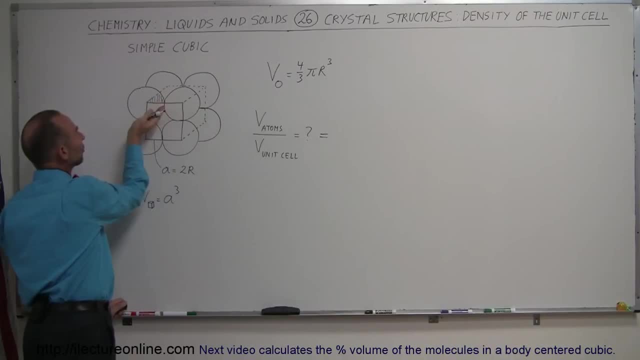 little corner right here, this little slice which is a ninety degree slice out of the bottom half of this atom. So if you think about you have the bottom half of the atom. you only take one quarter of the bottom half. that would only be one eighth of this cell. 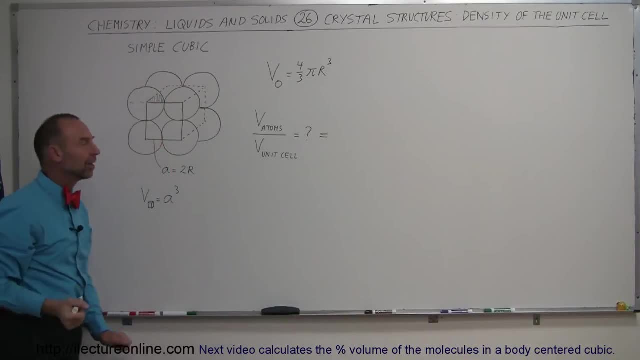 of this atom would be inside that cell. only one eighth of this one, one eighth of that one, one eighth of this one, one eighth of this one, this one, this one and one in the back that you can't see. Well, actually you might be able to see a little bit of it, but it's hard to see. 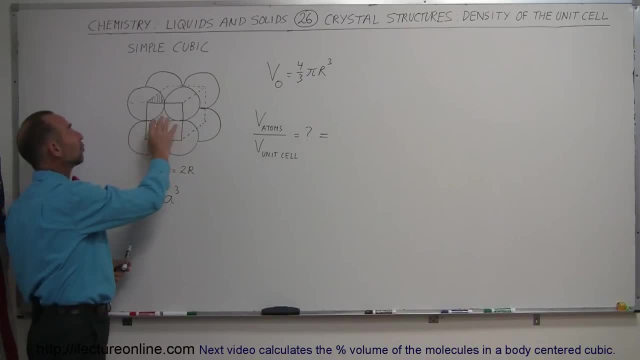 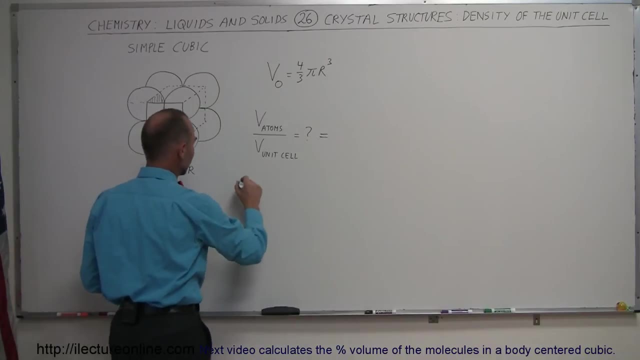 to draw in this particular fashion. So if there's eight times one-eighth of an atom, that means there's in total one complete atom inside that cell. So we have to determine the number of atoms in the cell and in this case, in this kind of packing arrangement, in the simple cube that is, 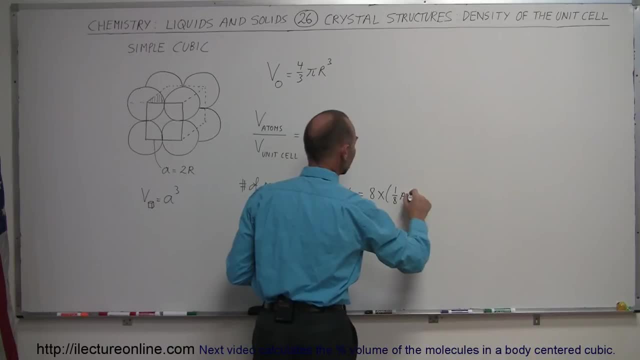 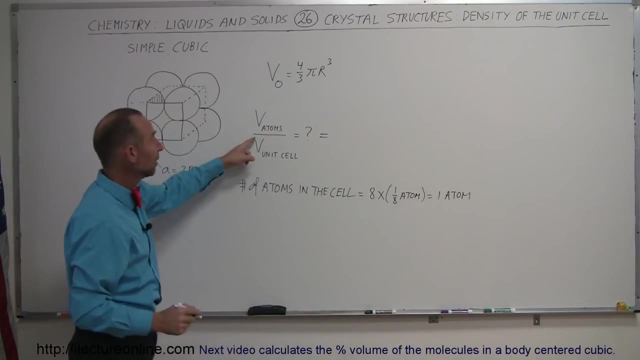 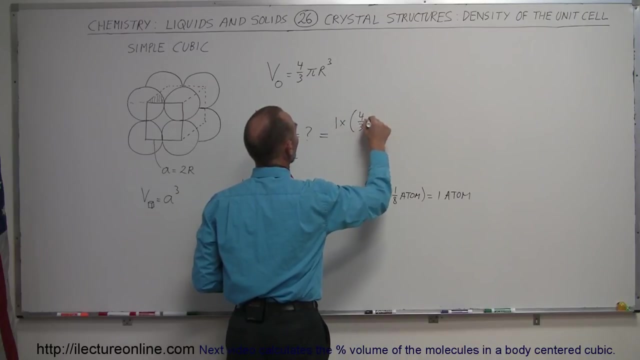 eight times one-eighth of an atom, which would mean it's one complete atom within that cell. So the volume then of all the atoms in the cell is the volume of one atom. so it would be one time four-thirds pi r cubed, and then of course the volume of the unit cell would be a cubed, and we 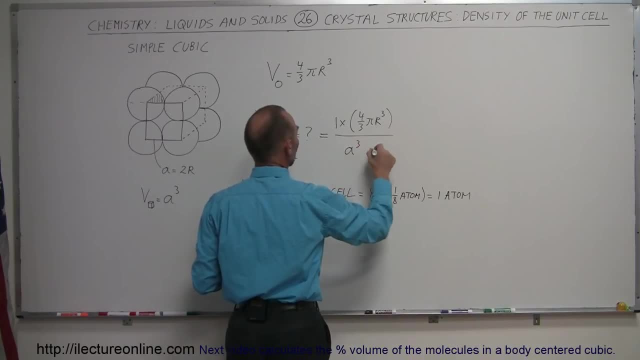 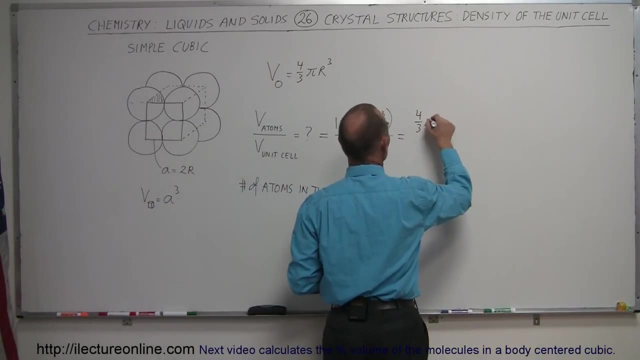 can go ahead and put that in there. So we have a cubed and, of course, a cubed. since a is equal to 2r, we can replace a by 2r, So this gives us four-thirds pi r cubed divided by 2r quantity. 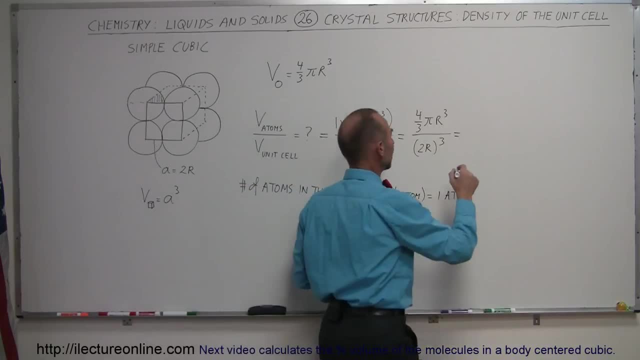 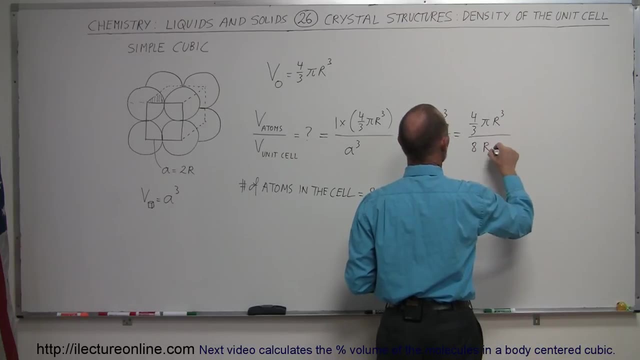 cubed. If we cube the denominator, we get the following: We get four-thirds pi r cubed divided by 8 r cubed. Right away we can see we can simplify some things here. The r cubed cancels out and the four divided. 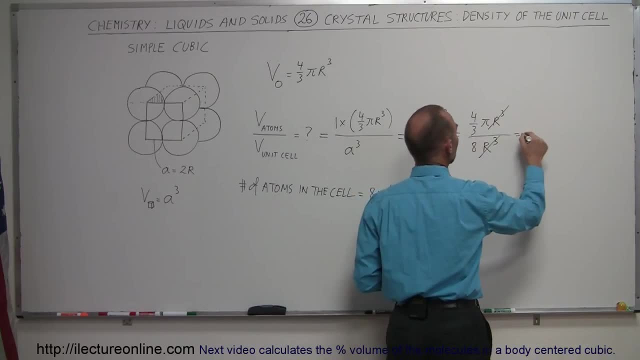 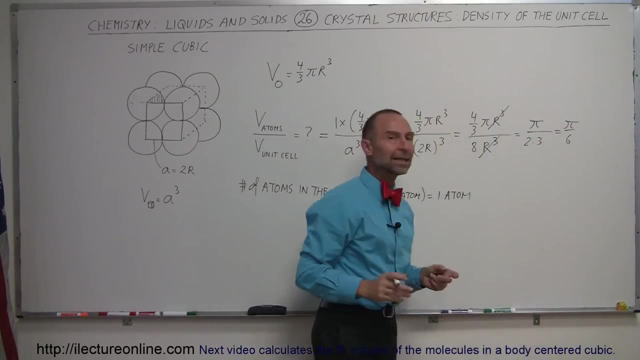 by 8 is one-half, and then we have a three in the denominator. so this would be equal to pi in the numerator divided by 2 times 3, or pi divided by 6.. That would be the percent or fractional volume.